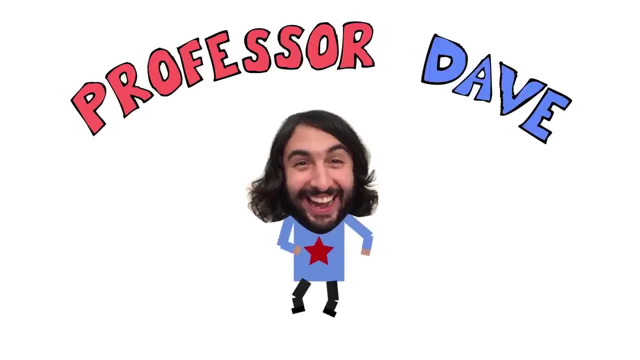 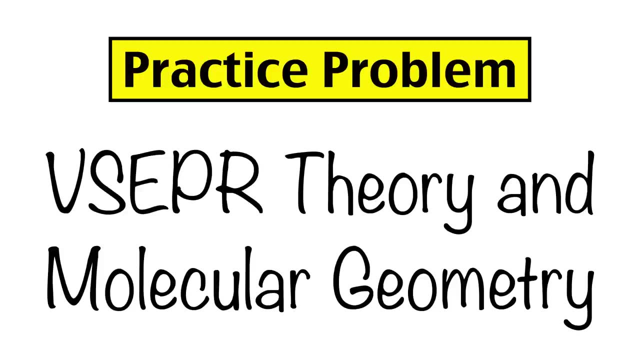 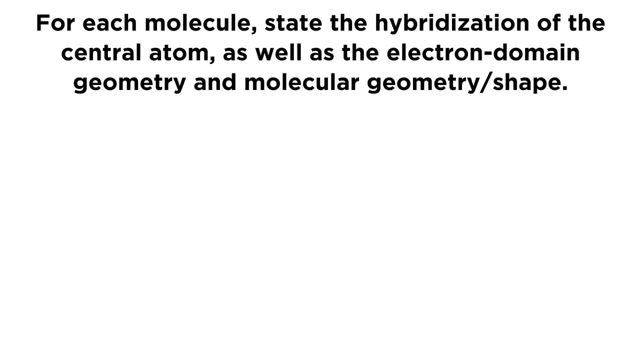 Let's take a look at a question regarding valence shell electron pair, repulsion theory and molecular geometry. So we're going to look at some molecules and for each molecule we need to state the hybridization of the central atom as well as the electron domain geometry. 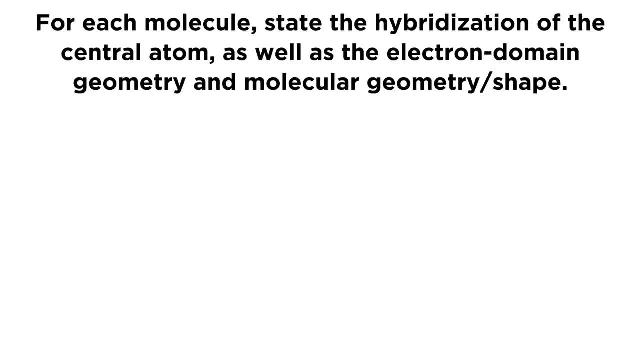 and molecular geometry or shape, which may be the same, but sometimes they are not the same, depending on lone pairs. So the molecules are NO3 minus or the nitrate ion NCL3,, CLF3, and XEF4.. So if this seems daunting, go ahead and check out some of my tutorials on Lewis. 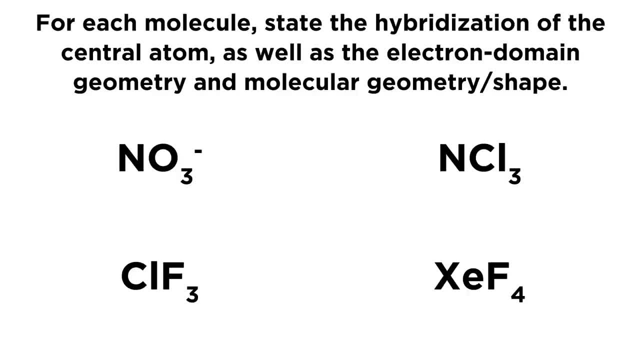 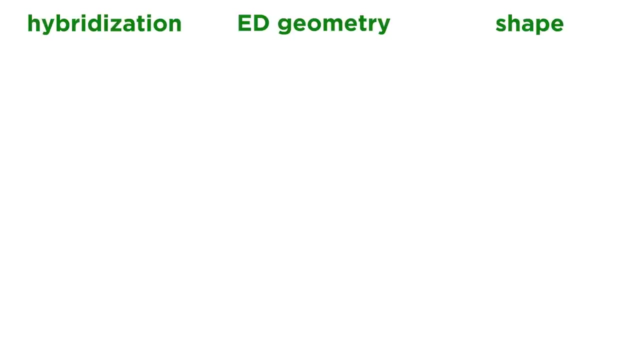 dot structures, as well as on VSEPR theory, and that will give you everything you need to answer these questions and you can give them a shot. So, once again, for each molecule, we need to state the hybridization of the central atom, we need to state the electron domain geometry and we need to state the shape or molecular geometry. 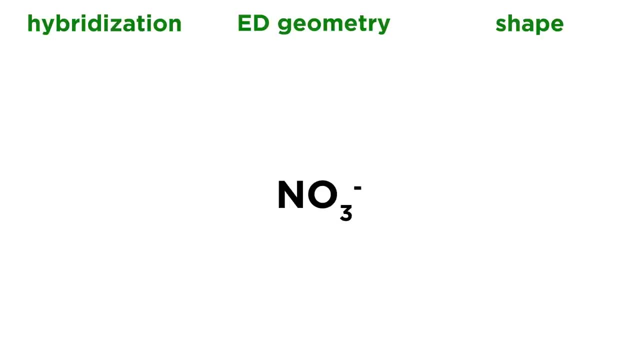 So first we have NO3 minus, Now that is the nitrate ion. so let's go ahead and draw the Lewis dot structure for this compound. So here it is. remember: nitrogen is going to have to have four bonds here, because it will have one bond each to two of the oxygens and then it will have to have two bonds a. 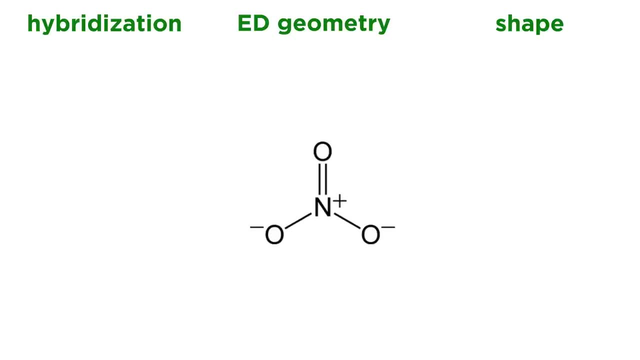 sigma bond and a pi bond to that third oxygen. So that means that two of the oxygens will be negatively charged and the nitrogen will be positively charged, because when nitrogen has four bonds it has a positive charge. So that is the Lewis dot structure for the nitrate ion. Now how are we going to get the 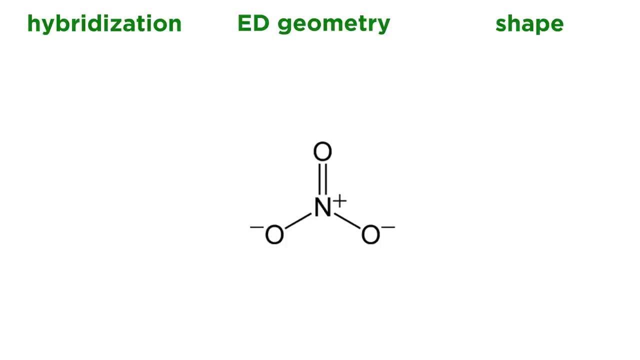 hybridization, We need to find out how many electron domains are surrounding the central atom. Well, the nitrogen atom is surrounded by three electron domains. Each of those oxygen atoms, or the covalent bond to those oxygen atoms, is considered an electron domain. So 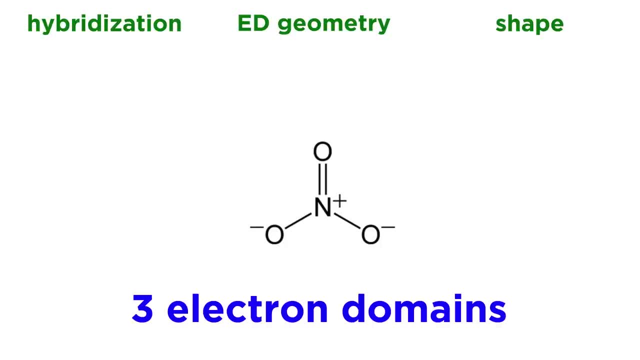 we have three oxygen atoms. we have three electron domains. Anytime, we have three electron domains. we have three electron domains. that means sp2 hybridization. it is going to need an s orbital and two p orbitals in order to hybridize them and make the hybrid orbitals necessary for this compound. so the hybridization. 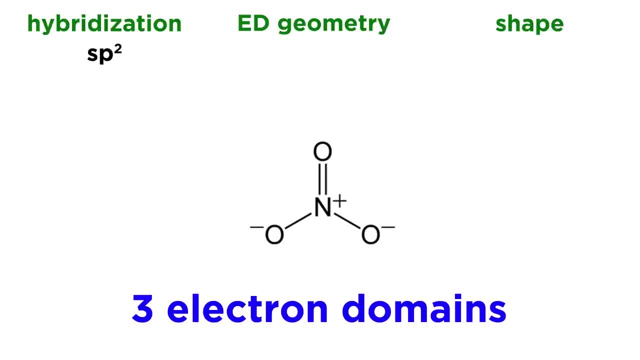 is sp2. anytime we have sp2 hybridization. the electron domain geometry is trigonal planar. those are always associated. so we have trigonal planar electron domain geometry. now, in terms of shape, we need to look at what those electron domains are, in this case these: 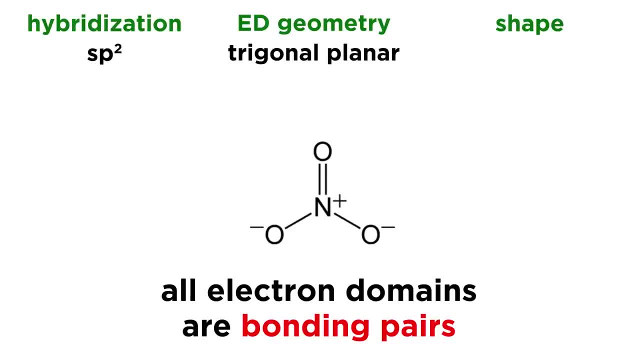 are all bonding pairs. all three electron domains are covalent bonds to oxygen atoms, so the shape will also be trigonal planar. whenever all of the electron domains are bonding pairs, the shape will match the electron domain geometry. it's only when some of them are lone pairs that the shape will 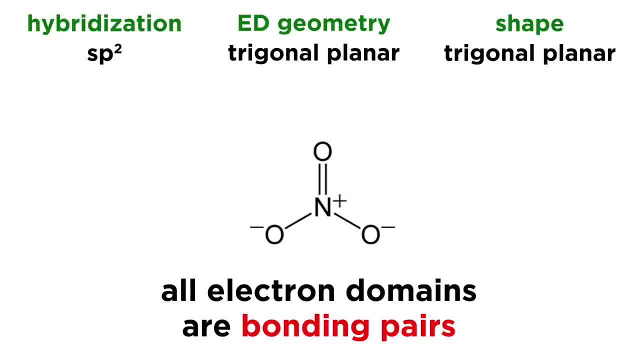 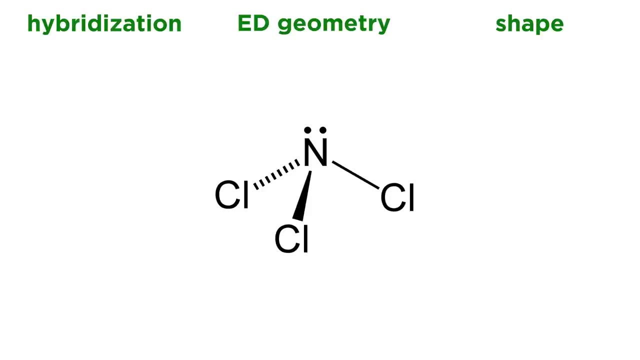 differ. so here the electron domain, geometry and the shape are both trigonal planar. okay, next let's take a look at nitrogen trichloride. so we have ncl3 once again. we're going to need that lewis dot structure to know what's going on. so nitrogen has five valence. 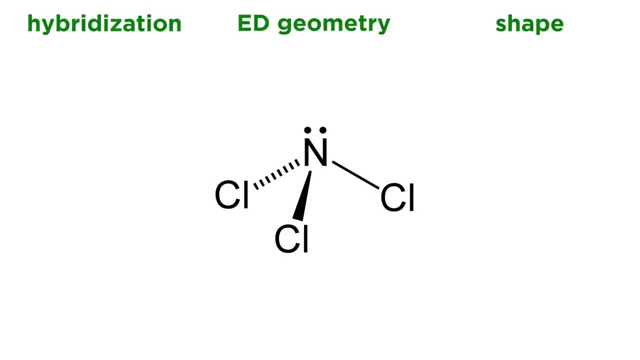 electrons. so it uses three of them to make the three covalent bonds to the three chlorine atoms, and then two are left over as a lone pair. so how many electron domains are surrounding the nitrogen atom? we have four electron domains. three of them are bonding pairs to the chlorine atoms and then 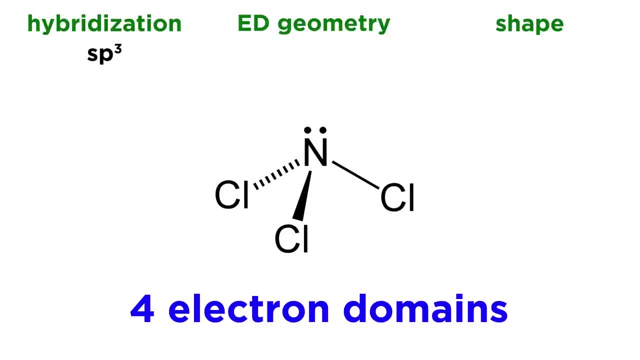 one of them is a lone pair and anytime we have four electron domains, that central atom is sp3 hybridized. you can count them up: we have s and three p's or s, p, p, p, that's four orbitals, that's four electron domains. that is sp3 hybridized. and anytime the central atom is sp3 hybridized. 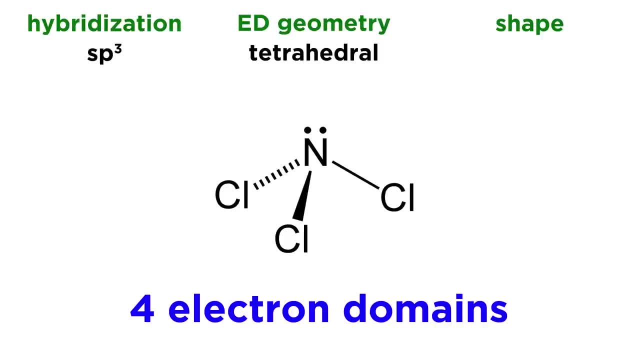 it will exhibit tetrahedral electron domain geometry. that will always be the case for the electron domain geometry of an sp3 center. so that's tetrahedral. now, in terms of shape, we have to look at what these electron domains are. so three of the electron domains are bonding pairs. right, we have. 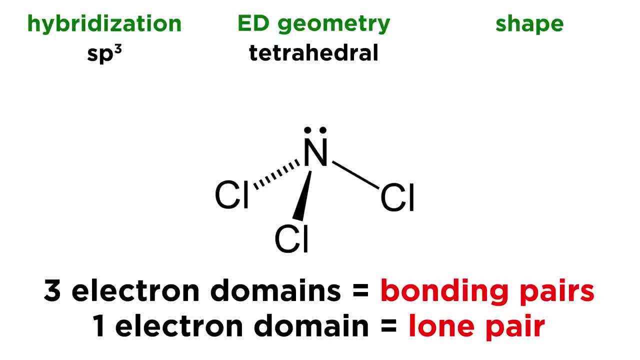 three bonds to three chlorine atoms, but that fourth electron domain. one of them is a lone pair. so we have one lone pair. that means that the shape will not be tetrahedral. so we have one lone pair. that means that the shape will not be tetrahedral. 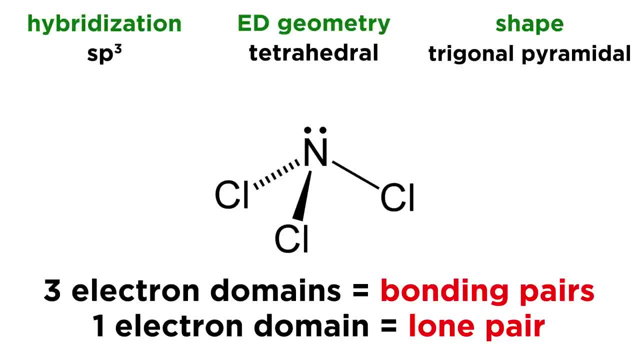 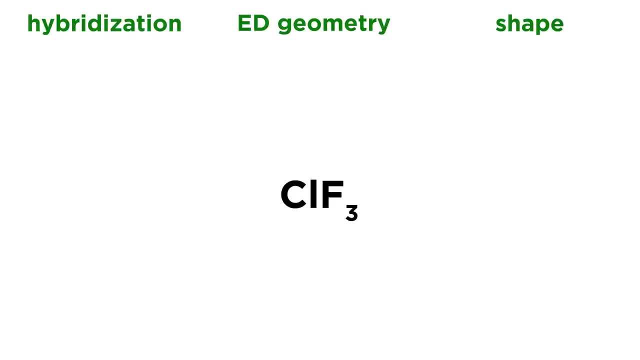 it will actually be trigonal pyramidal. so we can see the sort of pyramidal shape that is being formed by this molecule. so sp3: tetrahedral and trigonal pyramidal. now let's look at chlorine trifluoride. so this seems a bit odd, this interhalogen compound. but 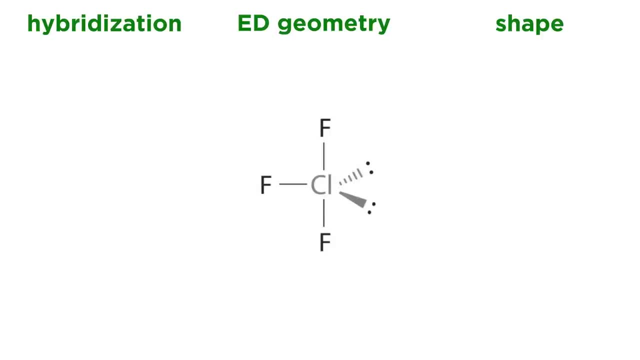 this does form and let's draw the lewis dot structure. so we've got that central chlorine atom and we've got three bonds to fluorine and one bond to chlorine and three bonds to tetrahedron, and then we've got two lone pairs. Now, this is the case because chlorine has seven valence. 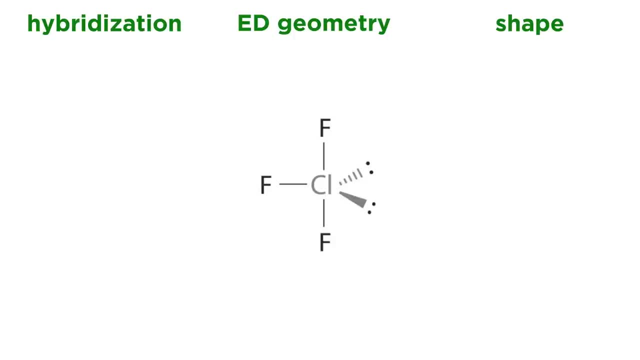 electrons. so if it uses three of them to make sigma bonds to fluorine atoms, it's got four left over in the form of two lone pairs. So that's the Lewis dot structure and that means we have a total of five electron domains. right, We have three bonding pairs to the three fluorine 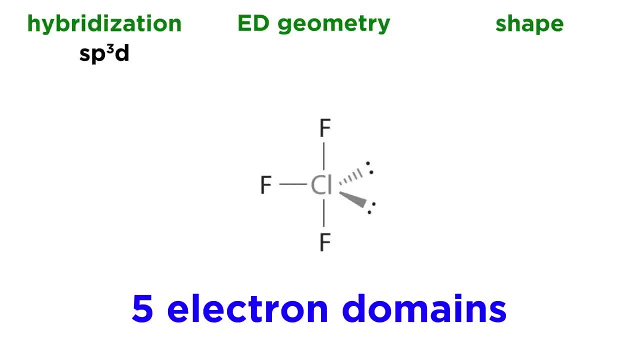 atoms and two lone pairs. So that is five electron domains: S P, P, P D, S P 3, D. The chlorine atom is S P 3, D hybridized and anytime we have a center that is S P 3, D. 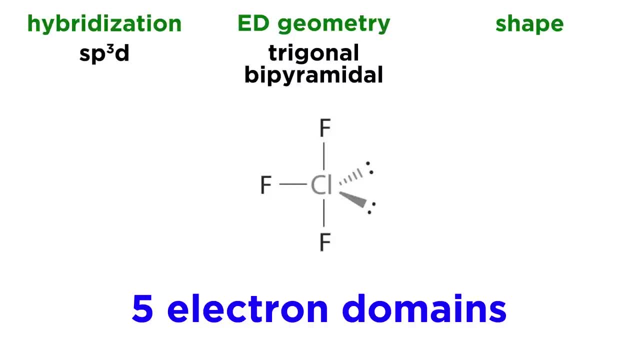 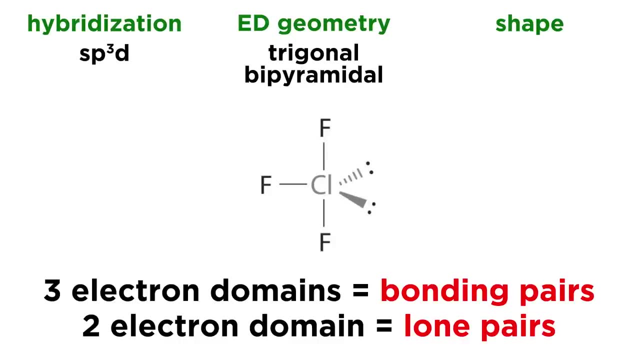 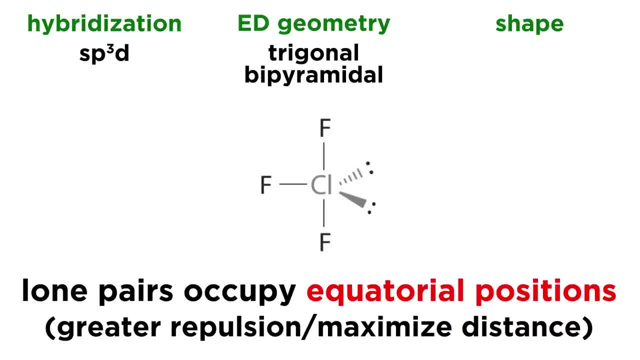 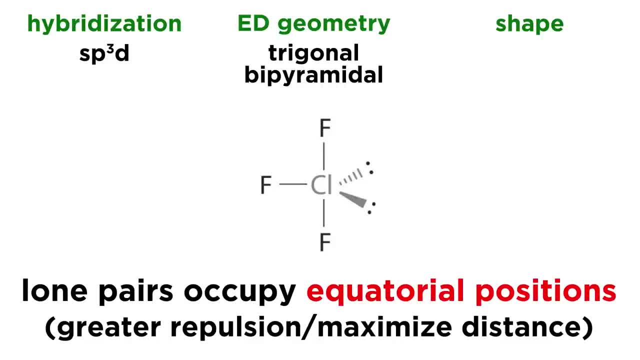 pairs have to occupy the equatorial positions. This is because lone pairs generate greater repulsion than bonding pairs, and so they want to be as far away from each other as possible. They want to maximize the distance, and the bond angles between those equatorial sites are 120 degrees. 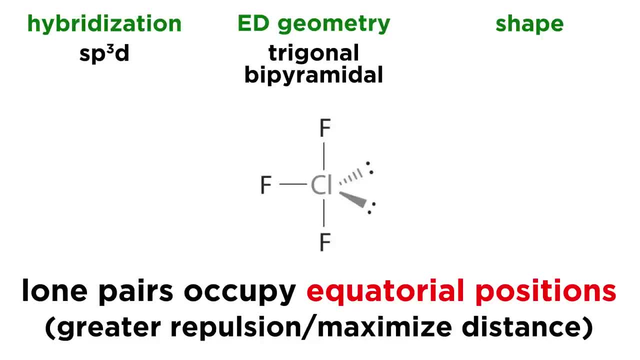 as opposed to 90, going up to the axial positions. So we're not going to put those lone pairs in axial positions, We're going to put them in the equatorial positions and that's very important because that informs the shape of the molecule If we put those lone pairs there. 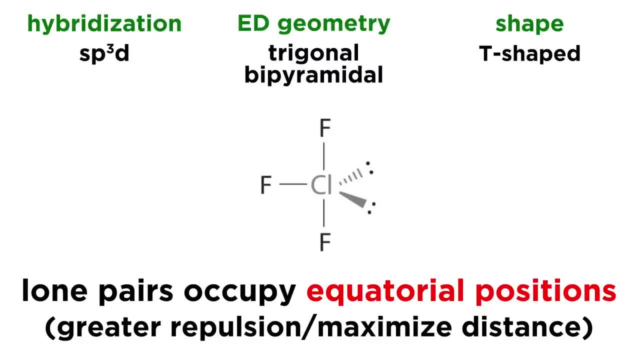 we are left with a molecule that is T-shaped. So T-shaped is going to be the shape here because of the position of those lone pairs. So we have S, P, 3, D trigonal bipyramidal. 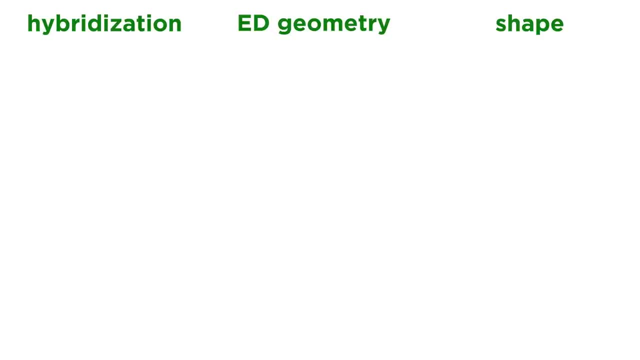 and then T-shaped, Okay. lastly, we have xenon tetrafluoride. Now, once again, we're going to have this loose dot structure with accurate geometry, So let's go ahead and put this xenon atom We're. 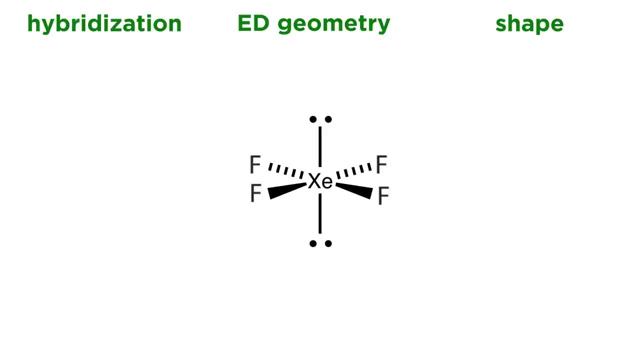 going to have four bonds to the four fluorine atoms. but don't forget, xenon has eight valence electrons. It is a noble gas, so it may be surprising that this can form covalent compounds, but indeed it can. And so xenon makes four sigma bonds to the four fluorines. It uses four. 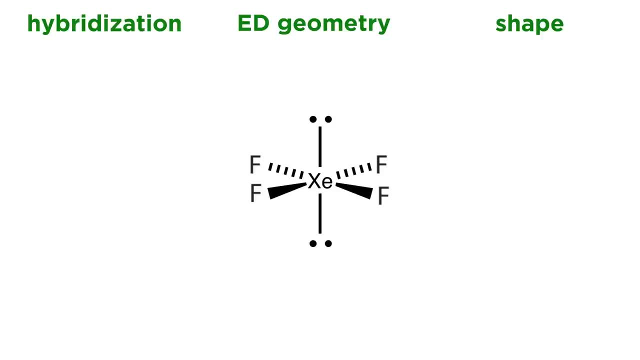 valence electrons to do so. That leaves four valence electrons left over to make two lone pairs, And so that is what this is going to look like. So we have six electron domains, four bonding pairs and two lone pairs, So S, P, P, P, D, D, S, P 3, D 2.. The xenon atom is S. 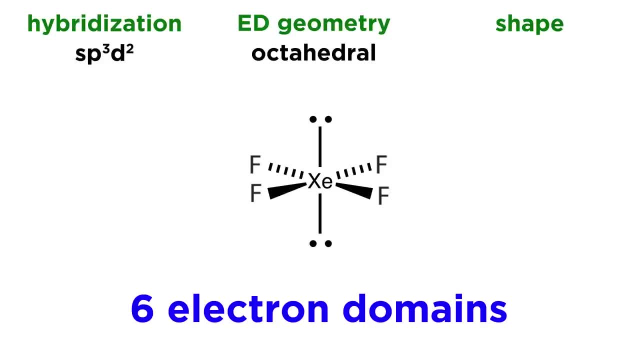 P 3, D 2 hybridized. and any time an atom exhibits S, P 3, D 2 hybridization, it is an octahedral center, So the electron domain geometry will be octahedral, regardless of how many bonding. 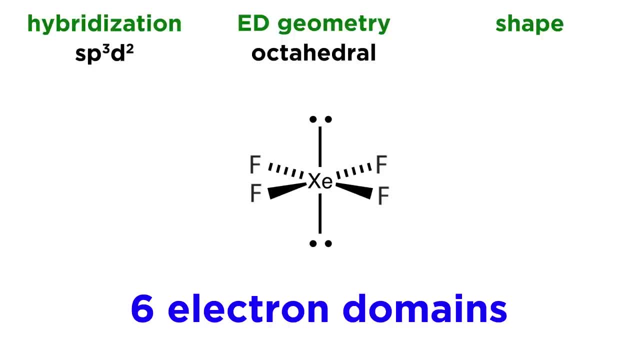 or lone pairs. So we have S? P 3, D 2 hybridized and any time an atom exhibits S P, 3, D 2 pairs there are. We have six electron domains. That is going to be S P 3, D 2 hybridized. 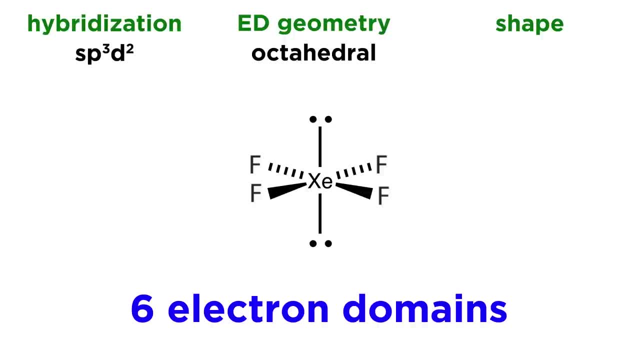 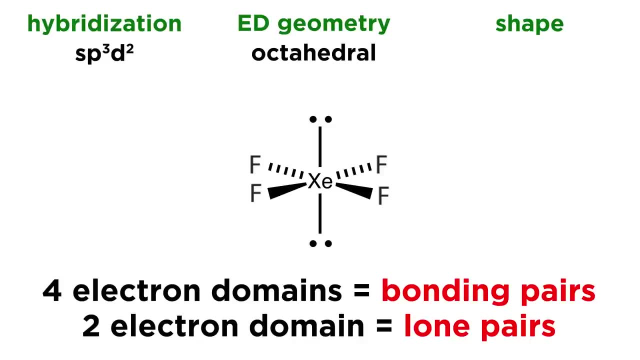 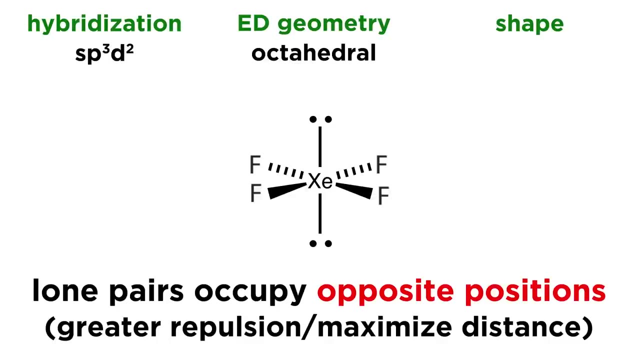 and always octahedral electron domain geometry. Now to assess the shape. As we said, we have four bonding pairs and we have two lone pairs. Now, once again, because those lone pairs exhibit greater repulsion than the bonding pairs, they're going to want to be as far away from each other. 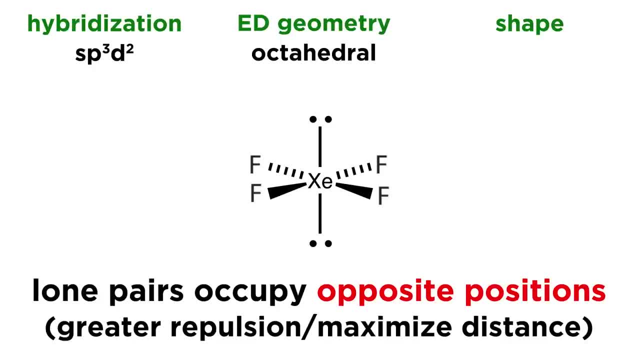 as possible. So they are going to occupy opposite positions. So wherever one lone pair, the other one has to be on the opposite side of that xenon atom, And so that's very important because that means the shape is going to be square planar. We can see those two fluorine.